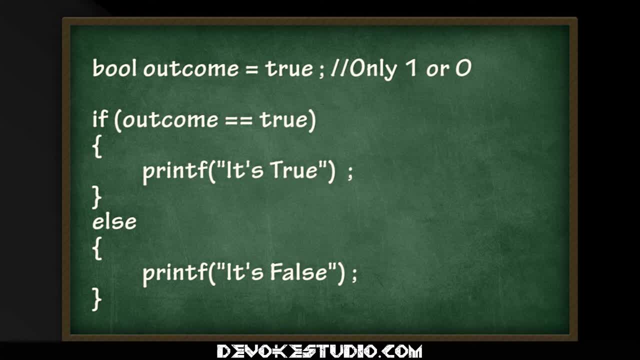 two values: 1 or 0, true or false. C does not have a official way of declaring the bool variable type, unlike other programming languages, but this is, of course, an introductory course to programming in general, Through which you will have a foundation of C. so be aware, in the future you will come across the bool. 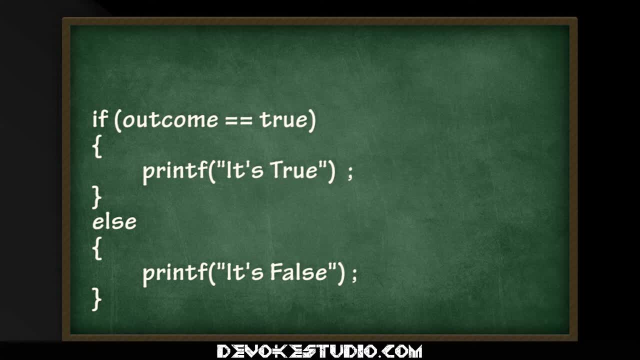 variable type, but the C programming language rather tests its true or false statements through conditional logic. For more information on this, have a look on the website at the chapter 2 hello world page, and a conditional statement is evaluated to be either true or false. But how do we? 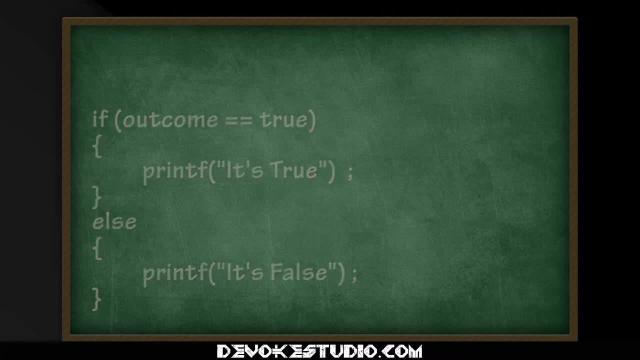 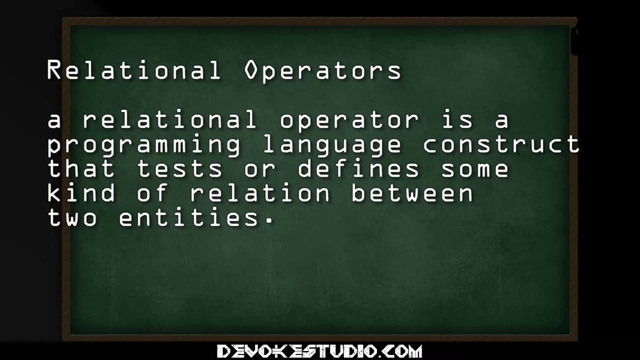 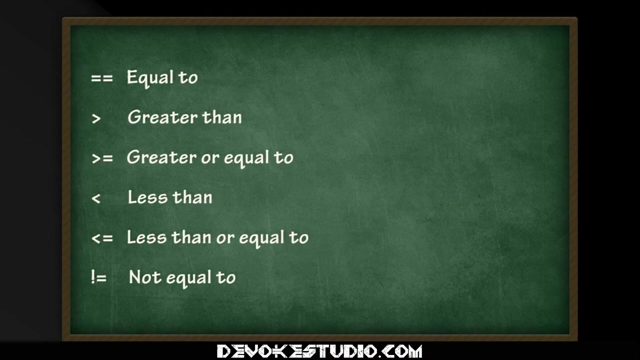 move past this. simple is equal to Well. we use things called relational operators. The first relational operator is the one you have already seen: two equal signs next to each other, and this is not the assignment operator. This is not what we use when assigning a value. This is one we use to 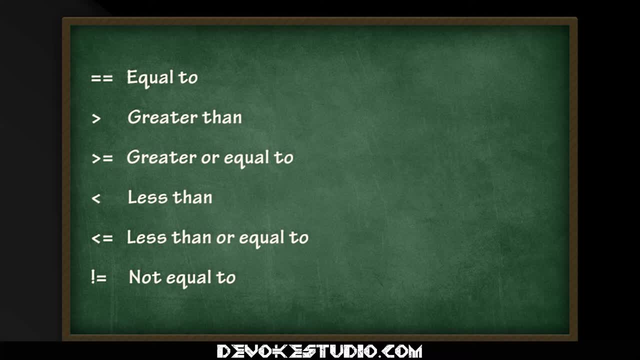 test whether it is equal. Instead, we say is equal to as a question. Next, is the greater than sign. You can remember this because in the West we read left to right and the widest point of this shape is on the left and the smallest is on the right. Is left larger than right? 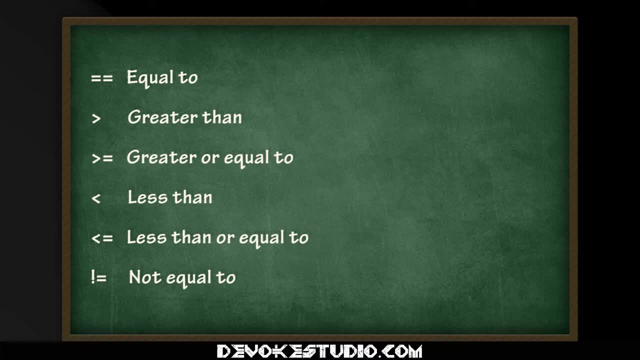 Next is the greater than or equal to sign. This means, rather than greater. we can also consider numbers that are equal to. Conversely, is the less than sign, where the item on the left is smaller than the item on the right. and, as you would expect, the less than or equal to sign. and then, finally, the not equal to sign, which evaluates. 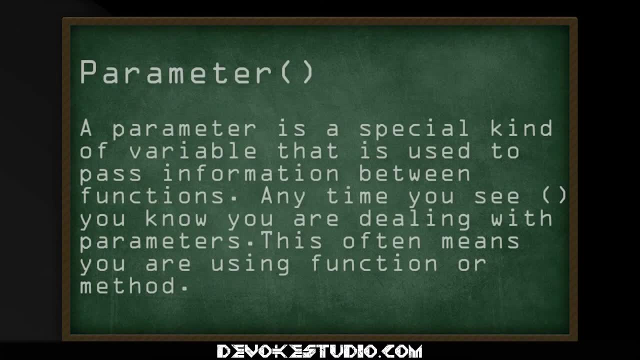 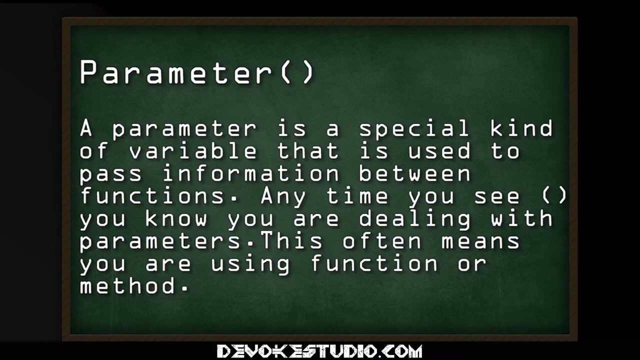 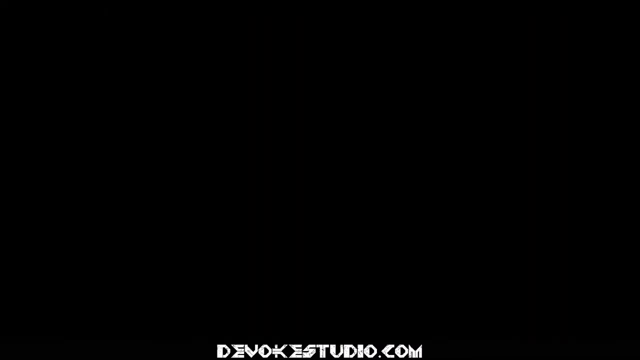 true when the left does not equal the right. The if statement is actually a form of something called a function. Remember any time you see two brackets like this: this is a parameter of the function or method, and in this case, the parameter of the if statement is the condition itself. So this is where you put your condition. 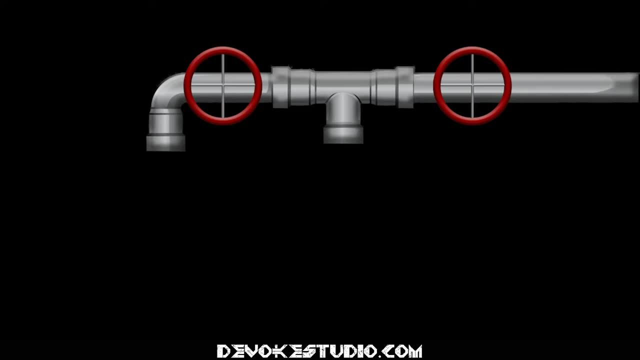 We can also think of conditional logic as the flow of data. So let's have one more demonstration, as the flow of data is very much how I want you to think of programs In general, how one is to control the data and information and its flow through the computer. 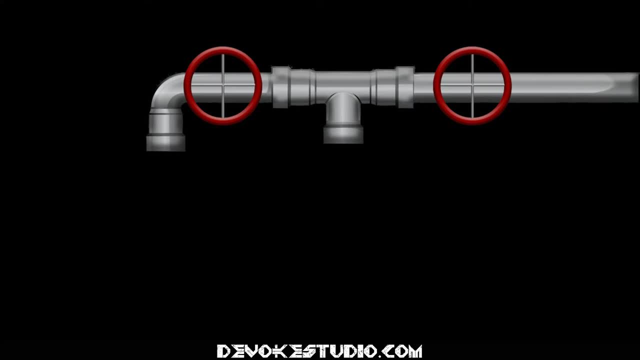 Here we have a simple pipe. As the wheel A turns, the gate is open, The condition for the liquid to flow was true, and when the wheel turns, the gate is closed, The condition is no longer true, but conversely else, if gate A is open, 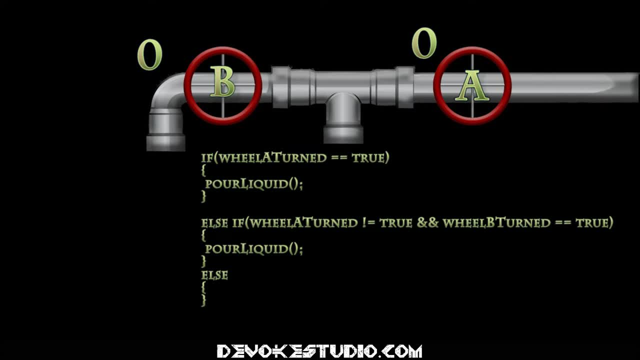 and when the wheel turns, the gate is closed. The condition is no longer true, But conversely else, if gate A is not open is closed and gate B is open, water will flow through the second pipe. This is a simple demonstration, but as you become more experienced through programming, you 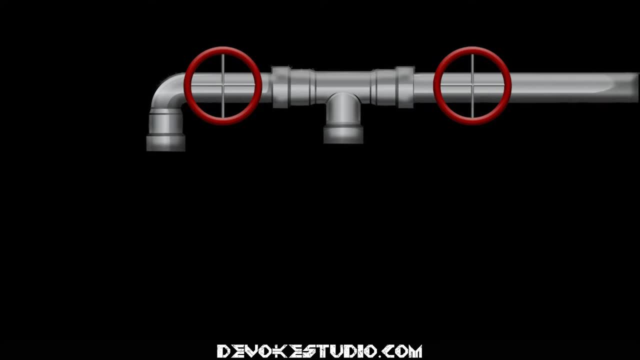 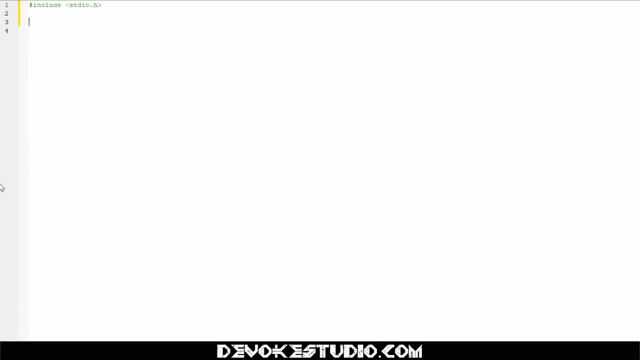 will start to interpret data as this flow. So let's practice with a little code. This program tool will be using the standard in-out library, as, of course, we will be gaining input from the user and simply open up an int main function and then begin prompting your user to input. 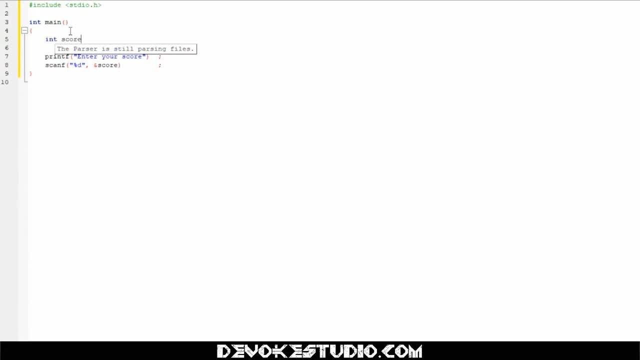 their score and make sure you use that address of operator when scanning for the input from the user. Now we print the score back to the user and start creating our if statements. If score was greater than or equal to 90 print. wow, you got an A Else if. 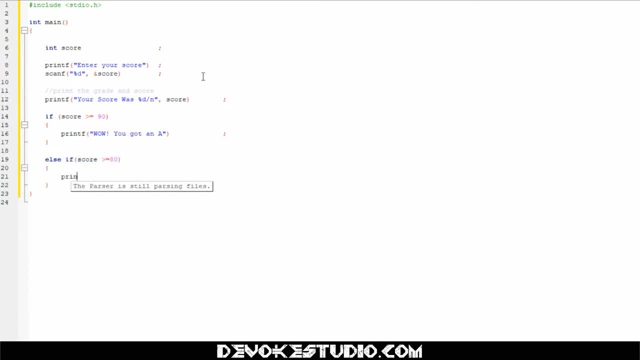 score was greater than or equal to 80 print: not bad. you got a B Else. if score was greater than or equal to 70 print, not bad. you got a C Else. if score was greater than or equal to 60 print: okay, you got a D Else print. well. 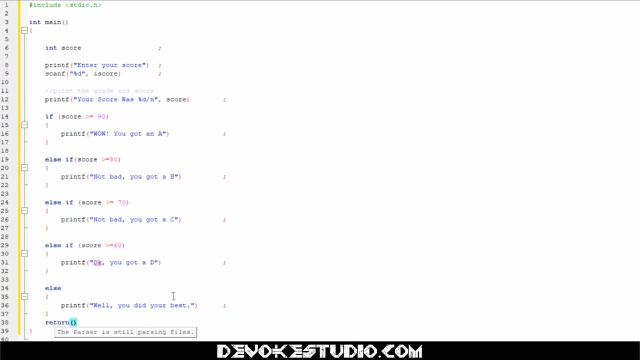 print- You did your best- Return and, of course, return 0, as we are using an int. So let's run our program and let's see what it looks like. Let's add some new line operators into all of these and now run to neaten up our code. Running our 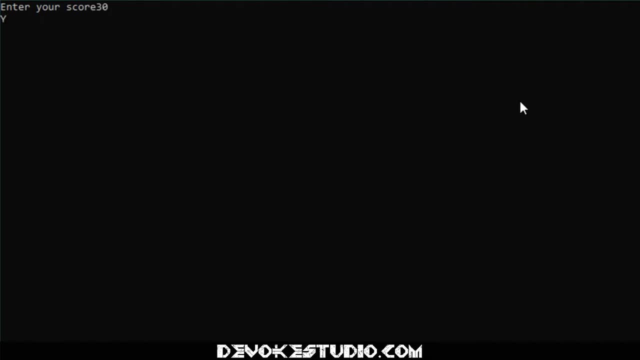 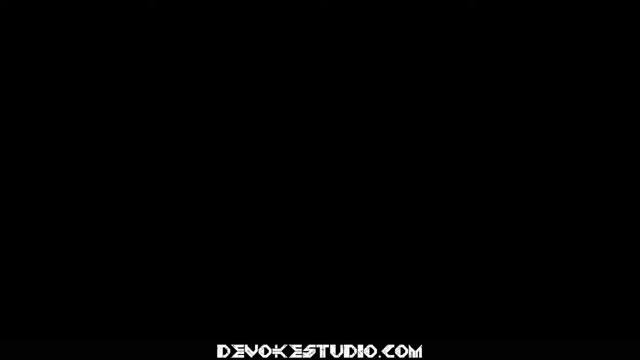 code. enter your score. let's try 30.. Your score was 30?? Well, you did your best. Try it again. enter your score 90. your score was 90. wow, you got an A. and with that simple demonstration, we can see how, just as I showed with the pipes and the voodoo doll- those 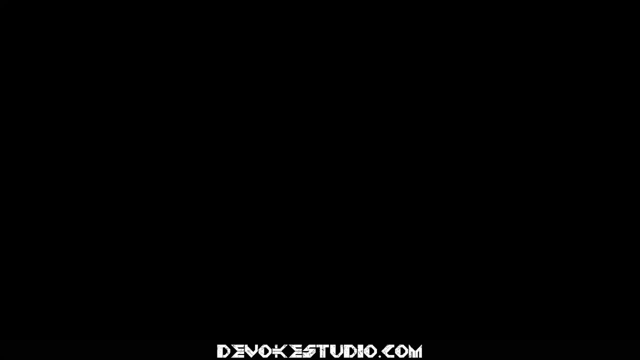 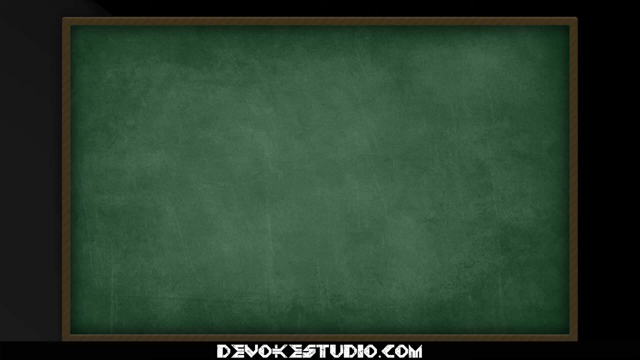 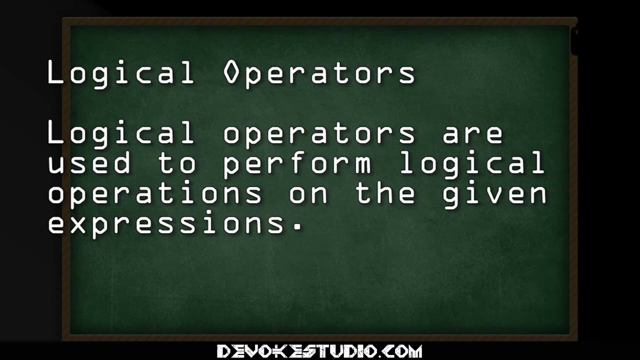 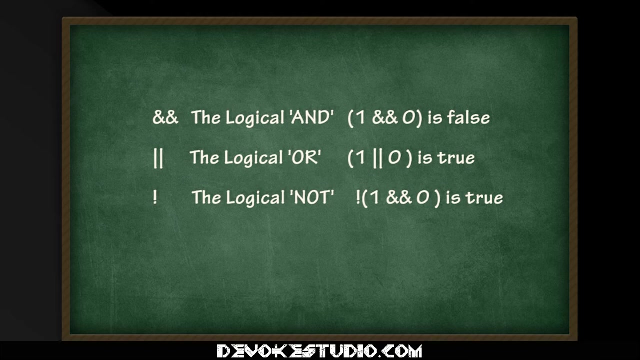 conditions change, changes the outcome of how the code was executed. so now this brings us nicely on to the logical operators. a simple explanation would be to say that these are the methods in which we construct our condition of what is true. in the C programming language, there are actually only three logical 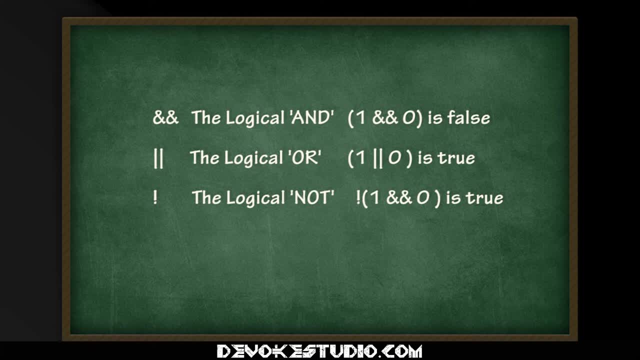 operators the and the logical or and the logical not. as you can see, one and zero evaluate to be false, as one and zero are not both true statements. if we use the logical or one or zero is true, as of course one is true and zero is false, then the statement is true. 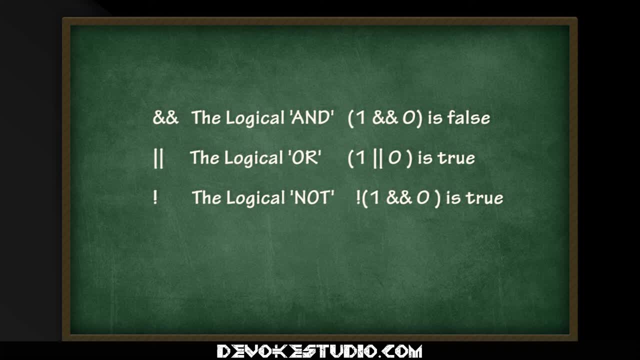 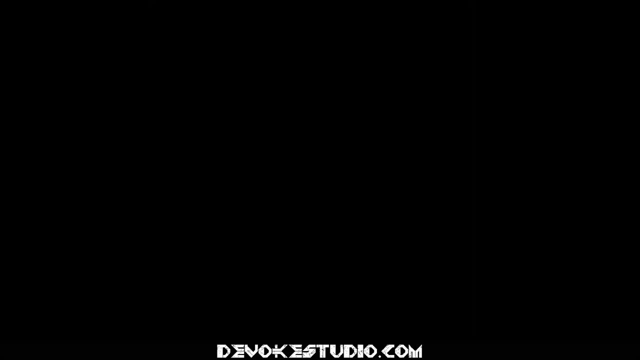 and the logical not one is not zero and therefore it is also evaluated to be true. so let's rewrite the code we had written before, using nested statements, but instead of this time use logical operators rather than if pricked by needle if needle is hot, as if pricked by needle and needle is hot, scream louder there. 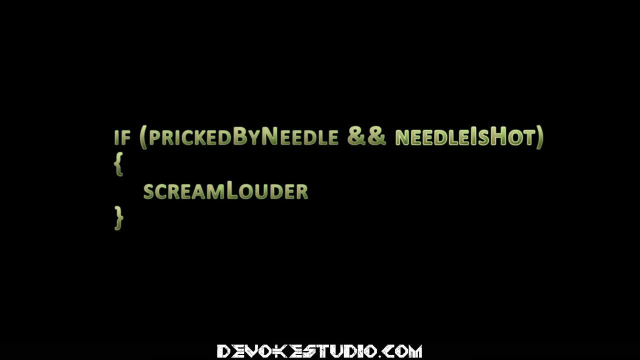 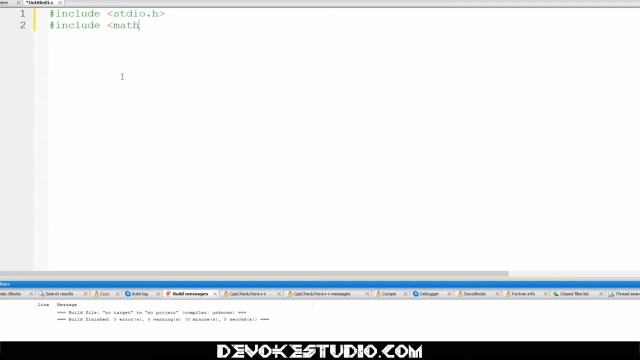 are advantages to both methods, of course. so here we begin by once again including the standard in out library, and also because we're going to be making a math program here, we're going to include the math library as well. even though it's not needed, it's good to get into the habit of practicing libraries that are 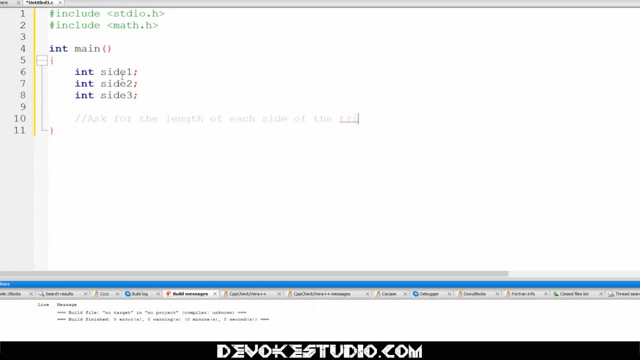 good for context. so we're going to be making a program here that has a lot of examples and I'm going to use the same thing here. we're going to have a variable that tells the user what kind of triangle they are looking at by having input of the three sides. so we have three variables, three int variables.